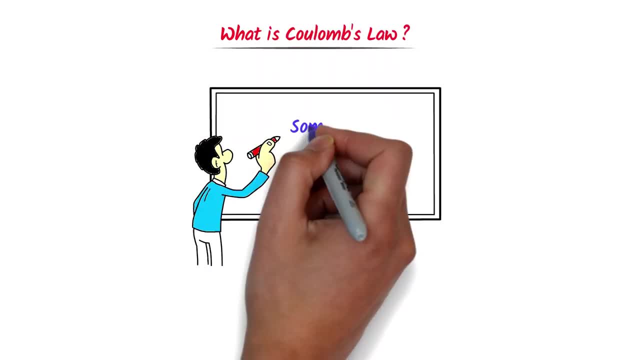 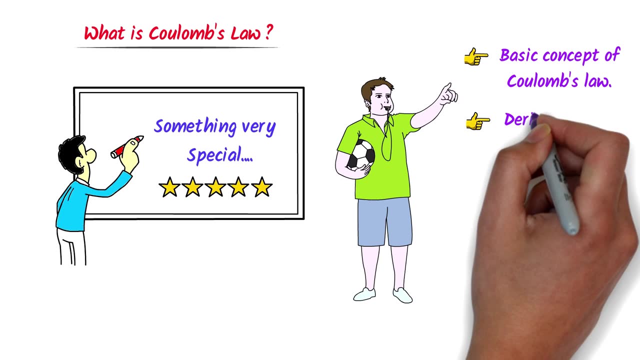 What is Coulomb's Law? Well, you will learn something very special in this lecture about Coulomb's Law. I will teach you the basic concept of Coulomb's Law, derivation of Coulomb's Law, bonus questions: best and easy explanation of writing Coulomb's. 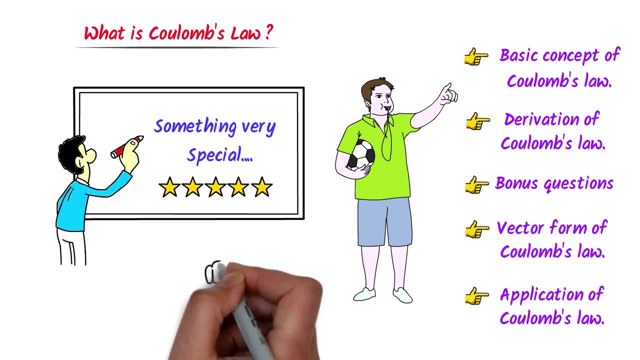 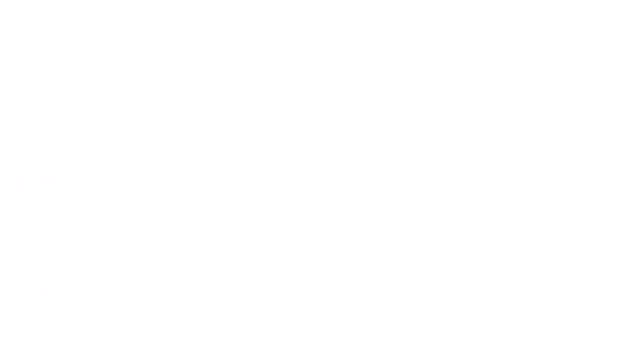 Law in vector form, applications and numericals. So watch this lecture till the end and you will learn something very awesome. Firstly, let me quickly revise the concept of forces between two charges. We all know that, like charges repel. For example, consider two positive. 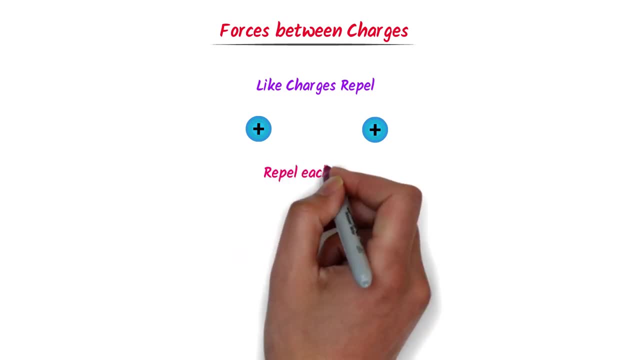 charges. We all know that they both repel each other. Now, in physics we do not say that they repel each other. Rather, we say that they experience repulsive force. Here, if I ask you that, how can you draw the direction of repulsive forces? 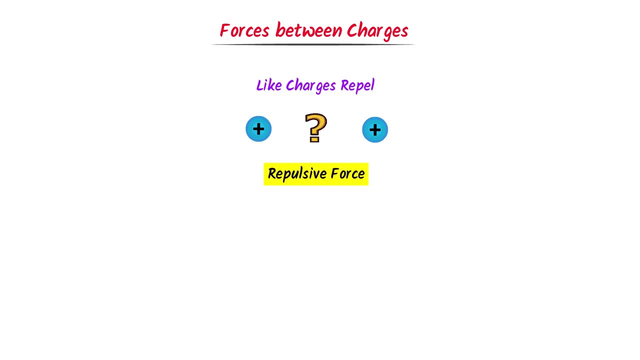 can you draw it? Well, many students do not know it. Let me draw it. This charge experiences repulsive force in this direction and this charge experiences repulsive force in this direction. So remember that there are two repulsive forces. Similarly, consider two negative charges. We know that. 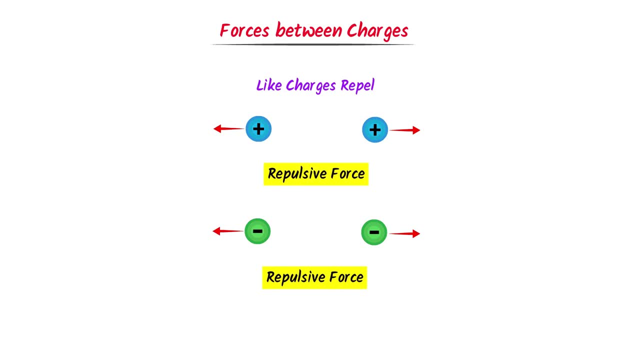 they also repel each other because they are like charges. So here again two forces, these act on two charges separately. Secondly, we know that unlike charges attract. For example, consider a positive charge and a negative charge. Now in physics we do not say that they attract. 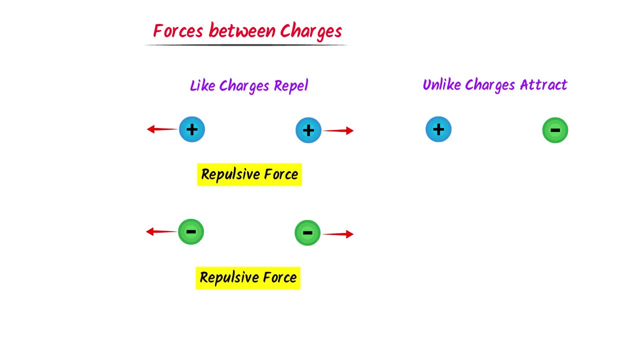 each other. Rather we say that they experience attractive force. In case of attractive forces, we draw them like this. So remember that attractive forces are different from positive forces. So remember that attractive forces are different from positive forces. So remember that attractive 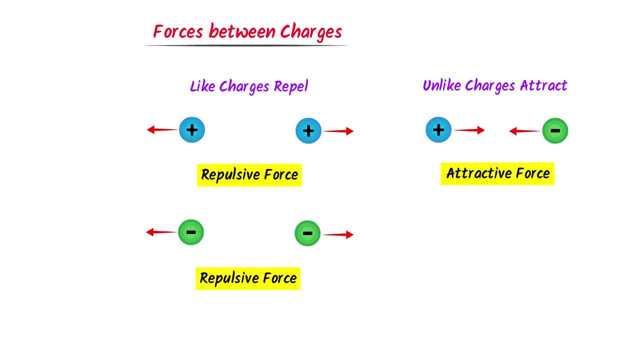 Attractive force are also two forces between two charge. Now here comes the most important question: If I ask you how much repulsive force exist between these two charge, or how much attractive force exist between these two charge, How can you calculate it? 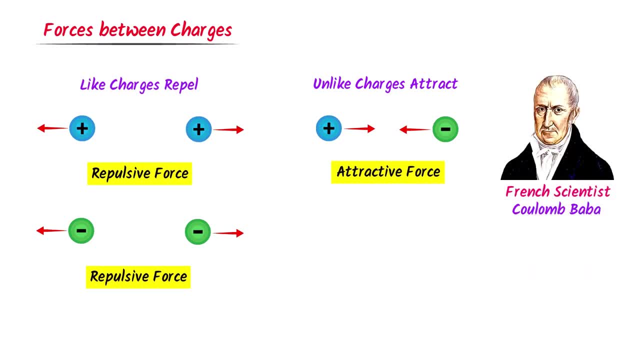 Well, it was first French scientist, Coulomb Baba, who successfully calculated this repulsive force between unlike charge and attractive force between like charge. He put forward his famous law, which we call Coulomb's law. Thus, in simple words, Coulomb's law calculate the force of attraction or repulsion between, 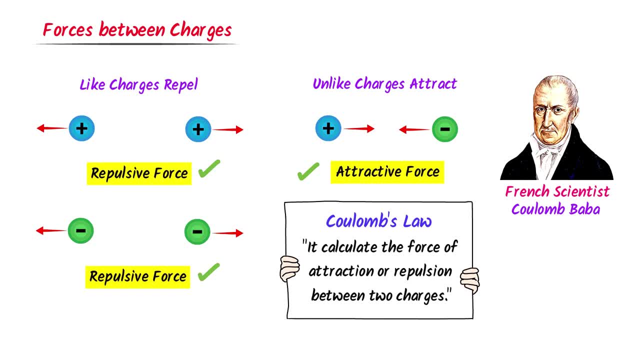 two charge. Let me repeat it In simple words: Coulomb's law: calculate the force of attraction or repulsion between two charge. Here let me teach you one important term Which is difficult for some students. We all know that we measure mass in kg. 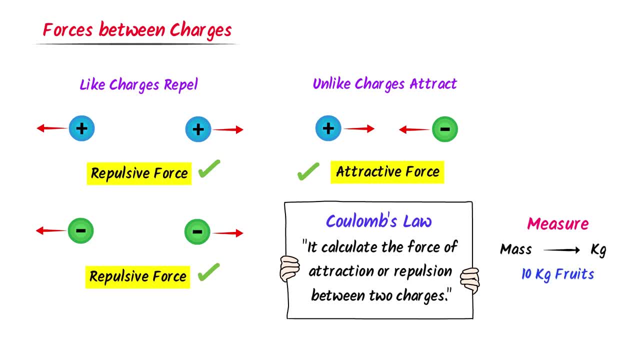 For example, we say that 10 kg fruits. Similarly, we measure charge in coulombs. For example, let the magnitude or size of this charge is 0.5 coulomb and the magnitude or size of this charge is 0.3 coulomb. 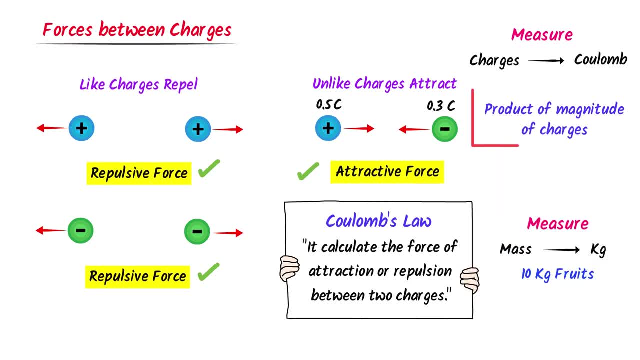 Now, if I say product of magnitude of charge, Can you understand it? Well, it means that we multiply the magnitude of these two charge and we write 0.5 into 0.3.. So note it down, this basic concept which some students are not understanding. 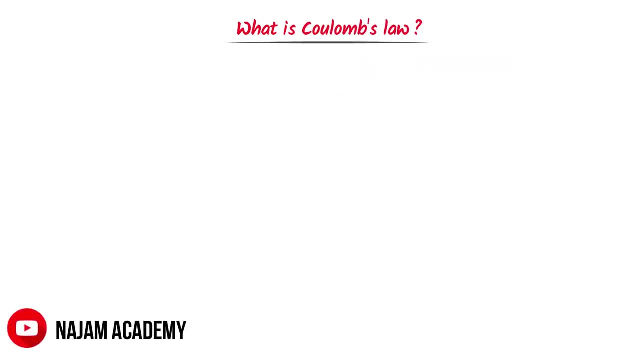 Now let me teach you what is Coulomb's law. Well, we have already learned that Coulomb's law calculate the attractive or repulsive force between two charge. Now consider two static charge or two point charge. at rest, Let I keep them and vacuum our air. 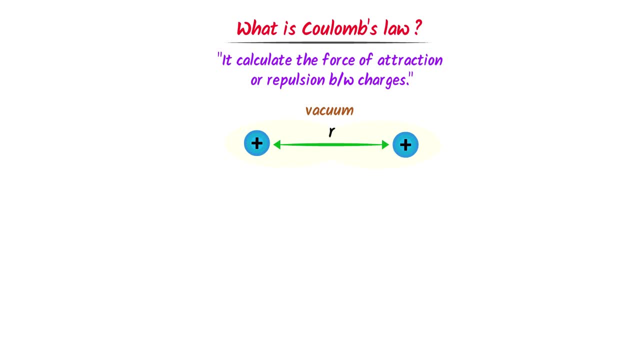 Let the distance between these two charge is r. The size or magnitude of this charge is q1 and the size or magnitude of this charge is q2.. We already know that there exist repulsive force between them. Now the question is, how much repulsive force? 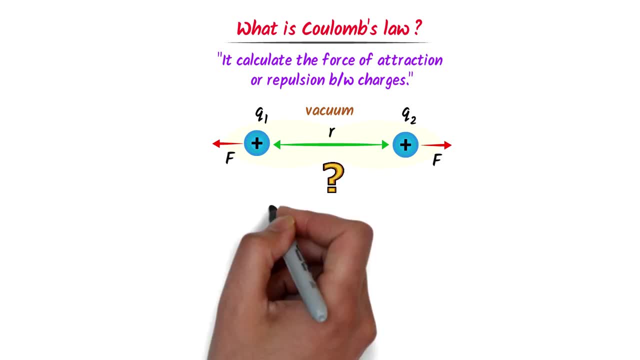 Well, according to coulomb's law, According to coulomb's law, the force between these two charges is directly proportional to the product of magnitude of charge. Let me repeat it: The force between these two charges is directly proportional to the product of magnitude of. 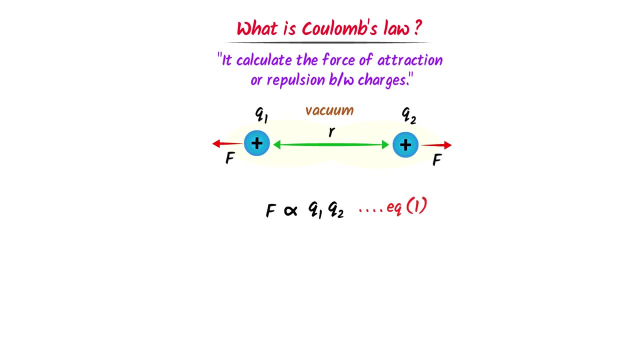 charge. Let. this is equation number one. Secondly, coulomb's law states that the force between these two charges is inversely proportional to the square of distance between them. Let me repeat it: The force between these two charge is inversely proportional to the square of distance between. 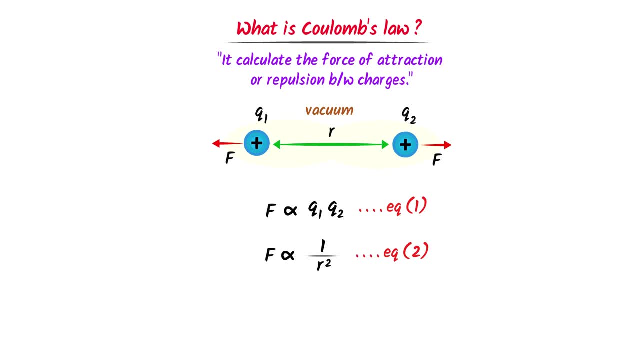 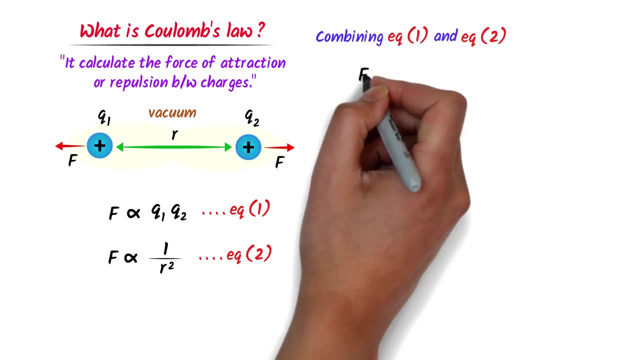 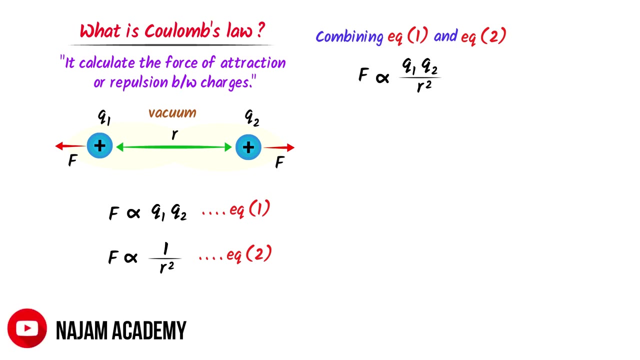 them Let. this is equation number two. Now listen carefully. I combine equation number one and equation number two. I write: f is directly proportional to the product of charge. Secondly, f is inversely proportional to the square of distance between charge. Here: 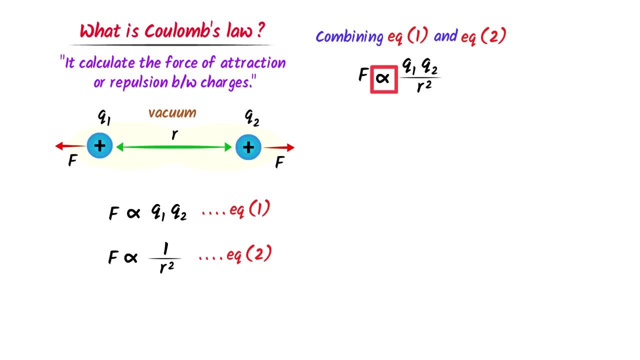 I am interested to remove the sign of proportionality. To do so I have to place a constant. So I write: f is equal to k into q1q2 upon r squared. This is known as coulomb's law. Here this k is known as coulomb's constant. 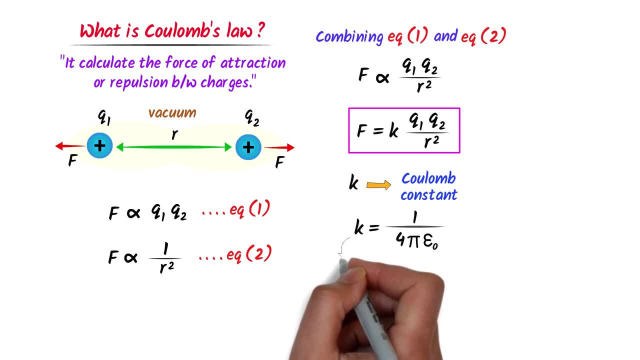 Our k is equal to 1 upon 4 pi epsilon naught. Remember that k is actually the property of a medium. Remember that k is actually the property of a medium. For instance, Here The medium is vacuum. In case of vacuum or air, the value of k is approximately equal to 9 into 10 to the power. 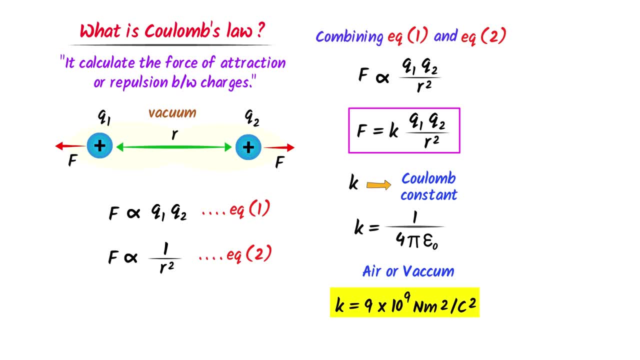 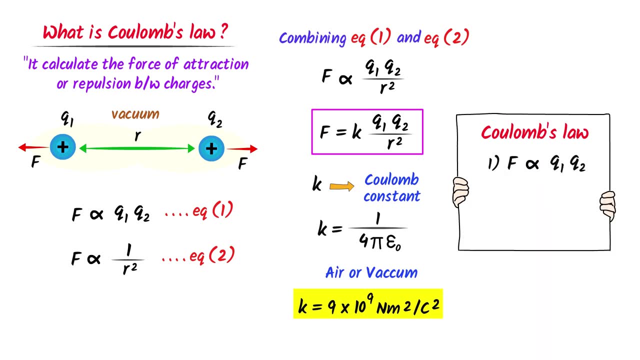 9 Newton meter squared per coulomb squared. Thus remember that coulomb's law depends on three factors: Product of magnitude of charge, square of distance between charge and the medium k in which charge are. keep Thus noted down all these important points. 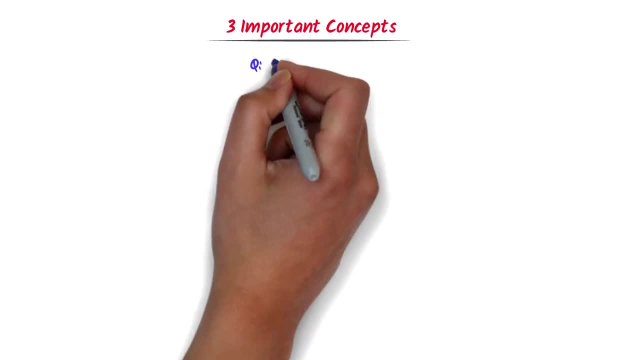 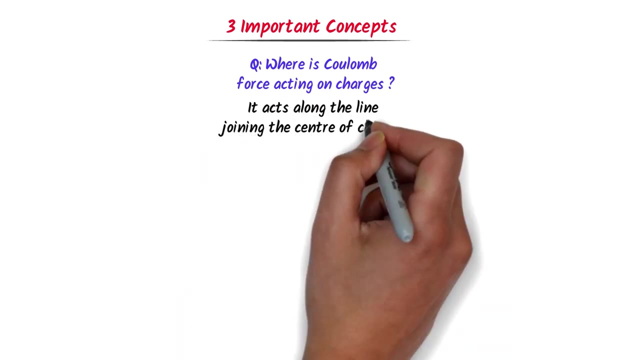 Now let me teach you three important concepts. Firstly, where is coulomb force acting on charge? Well, coulomb force act along the line joining the center of charge. For example, consider two charge. Here I draw a line between these two charge such that this line join the center of these. 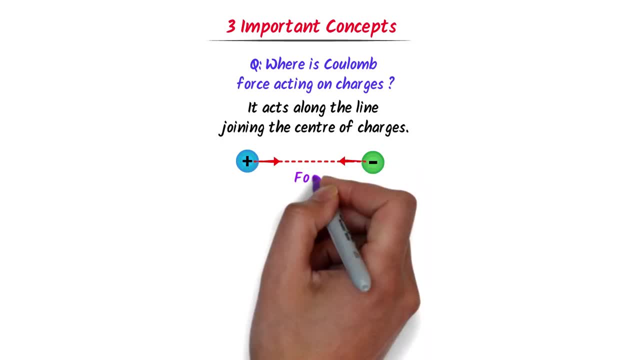 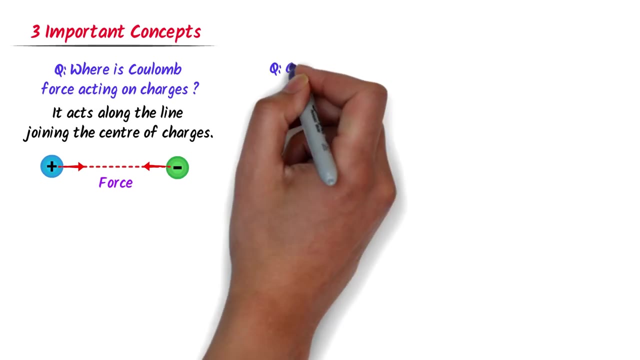 two charge: Coulomb force, either attractive or repulsive, always act along this line. Let me repeat it: The Coulomb force, either attractive or repulsive, always act along this line. Secondly, why Coulomb law is called inverse square law? 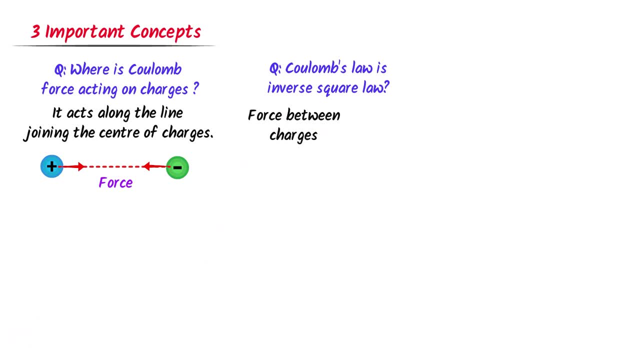 The simple answer is: force between two charge is inversely proportional to the square of distance between them. For instance, consider that I increase the distance between these two charge two times. As a result of this, the force will decrease four times between them. 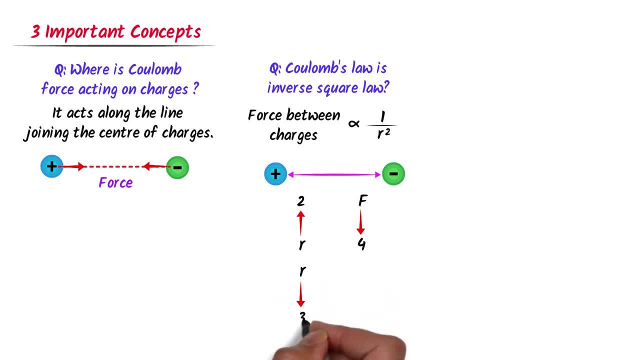 Secondly, consider that I decrease the distance between them three times. As a result of this, the force increase nine times between them. Therefore, we call it as inverse square law. Thirdly, what is meant by point change? Well, the simple answer is: the charge should look like a point in space from a larger distance. 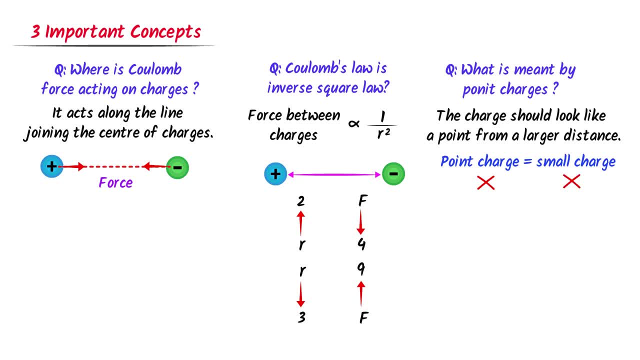 Point charge doesn't mean small charge, but it must be present at a larger distance. For example, consider stars in the sky. They are the best example of point charge. The stars are not small, rather they are extremely large. However, due to a larger distance, they are not small. 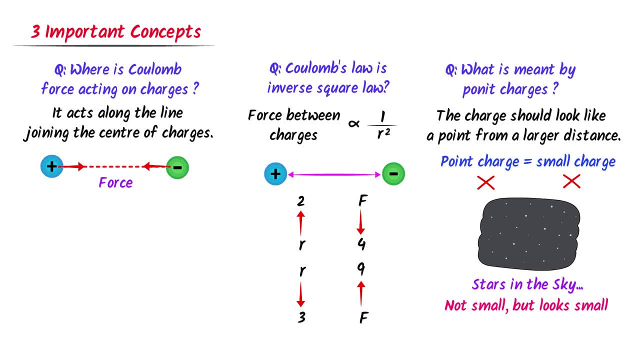 However, due to a larger distance, they are not small. However, due to a larger distance, they appear points in the sky. Therefore, remember that point charge means when charge appear points from a larger distance. Now let me teach you the most difficult concept of this lecture. 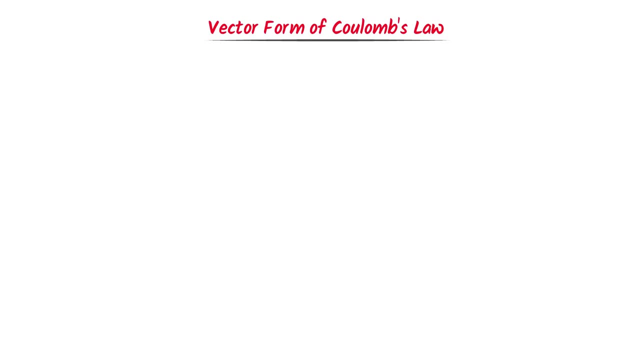 I mean writing Coulomb's law in vector form. I will teach you my personal method of writing it in vector form, which you will not find anywhere. Consider these two charge in the first part. In this part, Q1 charge will exert force on Q2 charge. 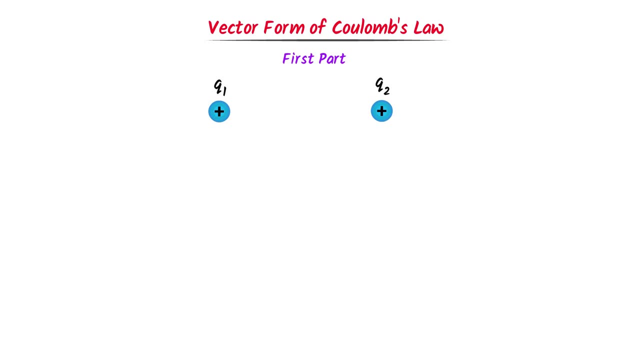 As a result, this Q2 charge is displaced. This Q2 charge experiences the force of Q1 charge in this direction. Now I call this force as F21.. Remember that F21 is force on Q2 charge due to Q1 charge. 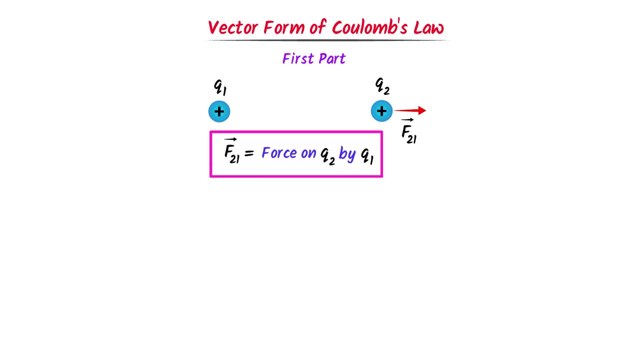 Let me repeat it: F21 is force on Q2 charge due to Q1 charge. Secondly, we know that, due to this force, the Q2 charge is displaced and this direction are away from the Q1 charge. So I call this displacement of Q2 as R12. 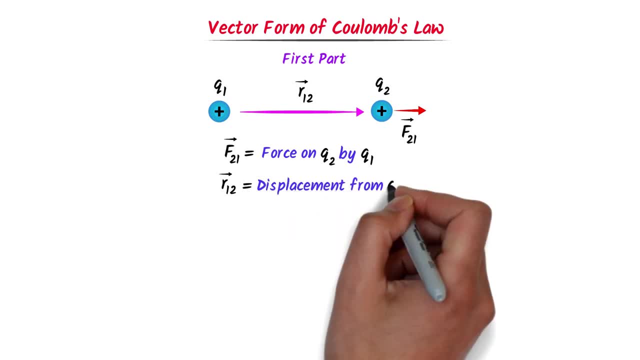 I mean R12 is the displacement from Q1 charge towards Q2 charge. Let me repeat it: R12 is the displacement from Q1 charge towards Q2 charge. Thus, remember that we have two parameters: F21,, which is the force on Q2 charge due to Q1 charge, and R12, which is the displacement from Q1 charge towards Q2 charge. 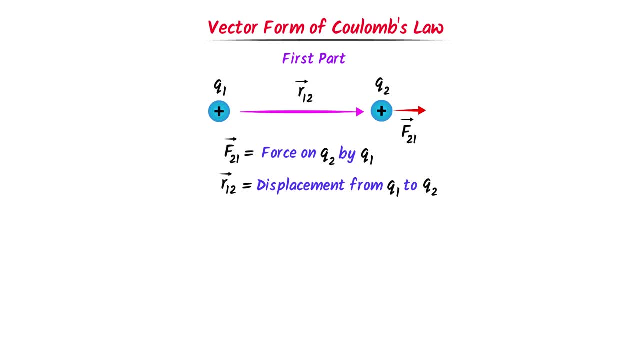 Now I will write vector for this force. We know that any vector like F is equal to its magnitude and unit vector. We know that the magnitude of F is k into Q1k, So the magnitude of F21 is equal to the magnitude of Q2 upon R2 into R12 hat. 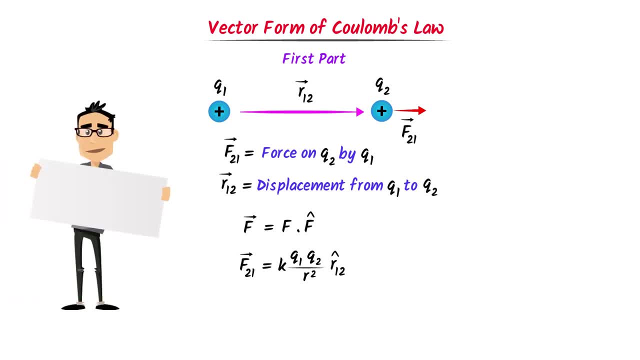 Now, this is how you learn in the traditional way in college. But have you ever asked your teacher that you are taking F21 force? you should put the unit vector of F21 hat. Well, let me explain it Here. I put the unit vector of F21 hat. 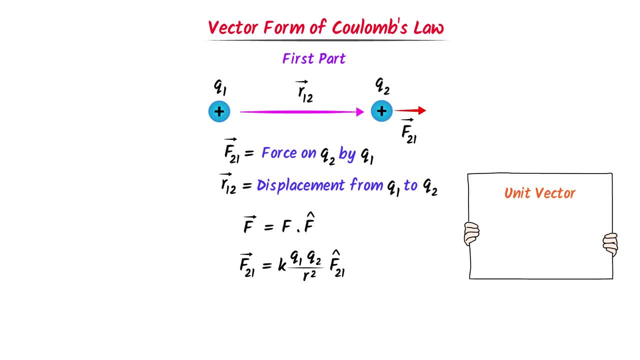 Now let me also explain the terminology of unit vector. Remember these two points about unit vector: Its magnitude is always 1 and it shows only direction. So the unit vector of F21 is F21 hat and its magnitude is 1.. 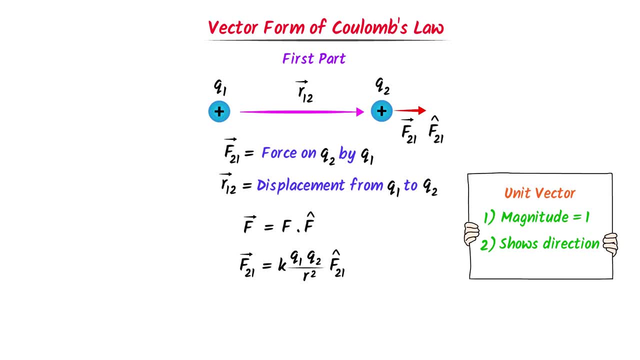 Similarly, the unit vector of R12 is R12 hat and its magnitude is 1.. Now listen carefully. Unit vector of F and unit vector of R are equal vector because they have same magnitude and same direction. Let me repeat it: Unit vector of F and unit vector of R are equal vector because they have same magnitude and same direction. 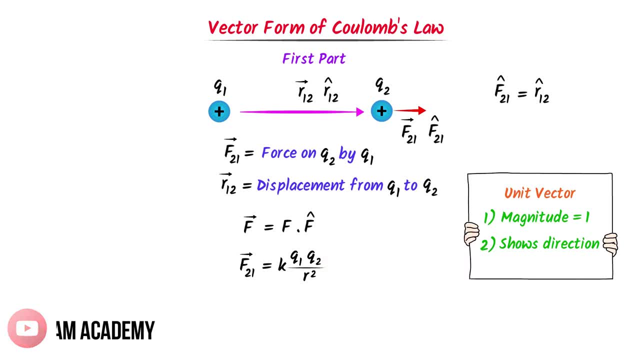 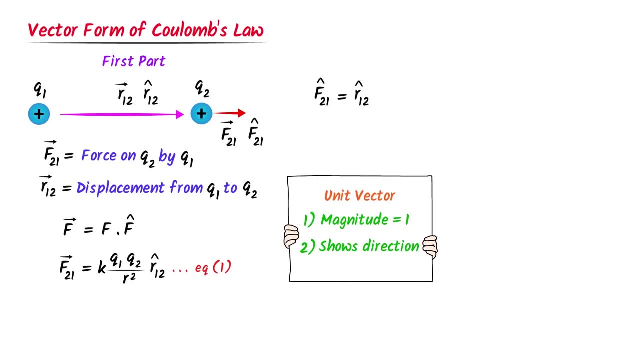 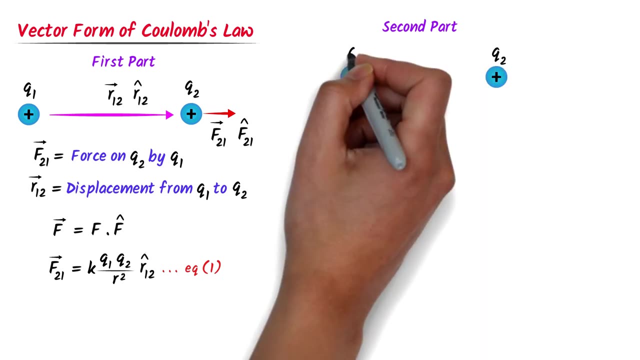 Thus, instead of this F21 hat, I can put R12 hat unit vector Let. this is equation number 1.. Now consider these two charts in the second part. Here, Q2 will exert force on Q1.. As a result of this, Q1 is displaced. 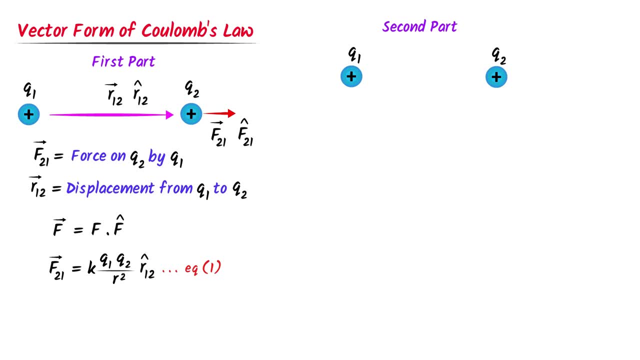 We already know that Q1 experiences force of Q2. We call it F12. Our F12 is the force on Q1 by Q2.. Secondly, this Q1 charge is displaced away from Q2.. We say R21 is the displacement from Q2 towards Q1. 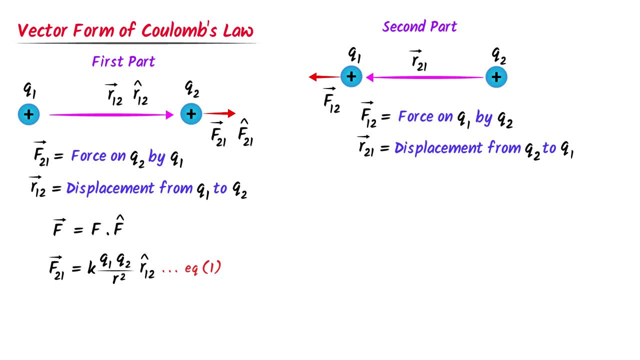 Let me repeat it: R21 is the displacement from Q2 towards Q1.. Now I will write vector form of this force. F21 is equal to K into Q1, Q2 upon R squared into F12 hat. We already know that the unit vector of F12 and R12 is the same. 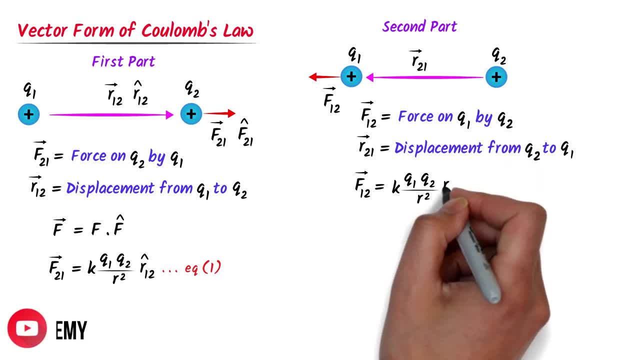 So instead of this, I write: R21 hat unit vector Let. this is equation number 2.. Now listen carefully. I take this unit vector R12 of equation number 1 and I write it here. Similarly, I take unit vector R21 of equation number 2 and I write it here: 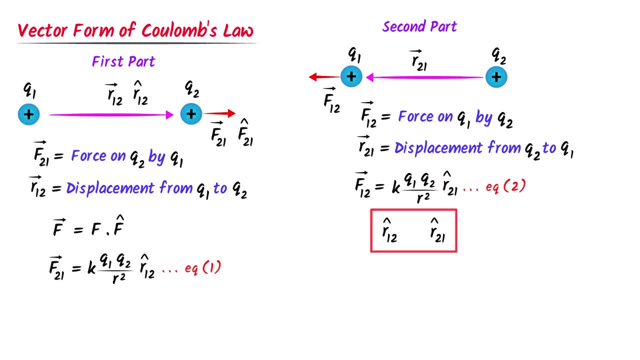 We know that the magnitude of unit vector is 1.. What about its direction? Well, the direction of R12 unit vector is towards right And the direction of unit vector R21 is towards left. So I write: R12 is equal to negative R21.. 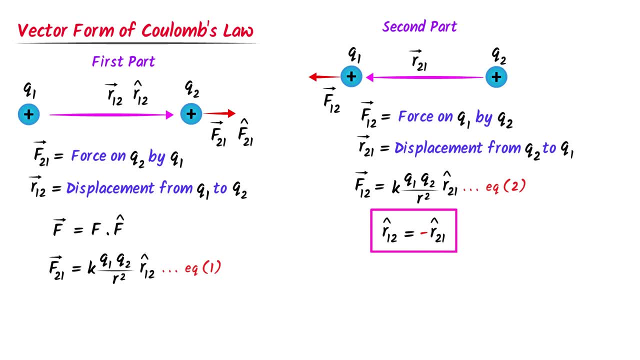 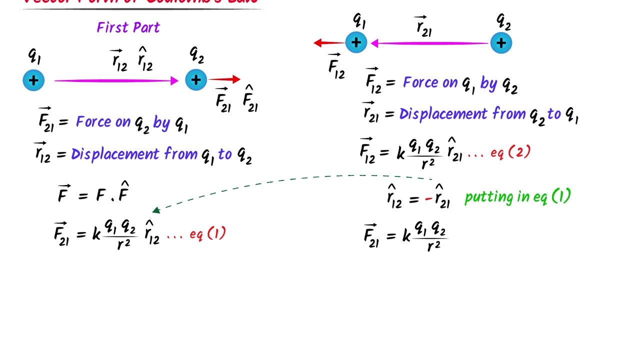 Remember that here this minus sign indicates opposite direction. Now I can put this unit vector in either equation, equation number 1 or equation number 2.. For example, I put minus R21 in equation number 1.. I write: F21 is equal to K into Q1, Q2 upon R squared into minus R21.. 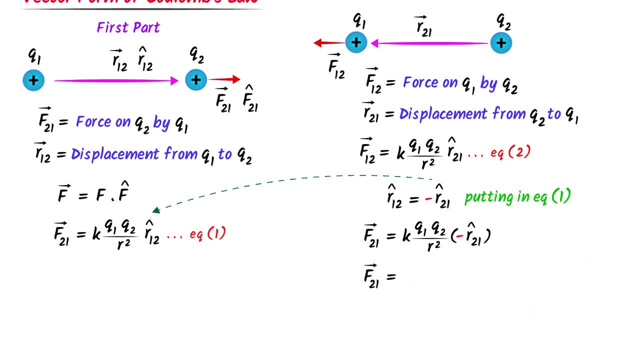 R. F21 is equal to. I bring the minus sign to the first position into K. into Q1. Q2 upon R squared into R21 hat. Now listen carefully. We can see that F12 is also equal to K- into Q1. Q2 upon R squared into R21 hat. 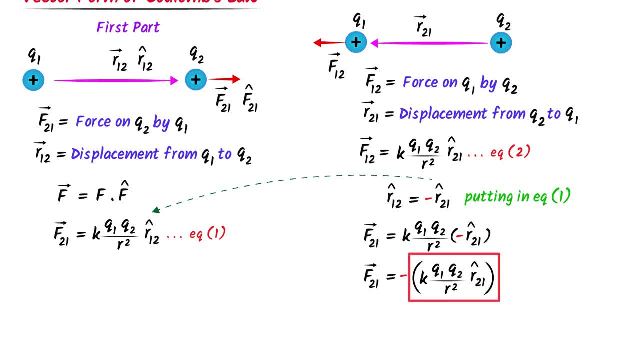 So instead of this I put here F12. Thus I get: F21 is equal to minus F12. It means that these two charts exert equal forces on each other in opposite direction. Let me repeat it: These two charts exert equal forces on each other in opposite direction. 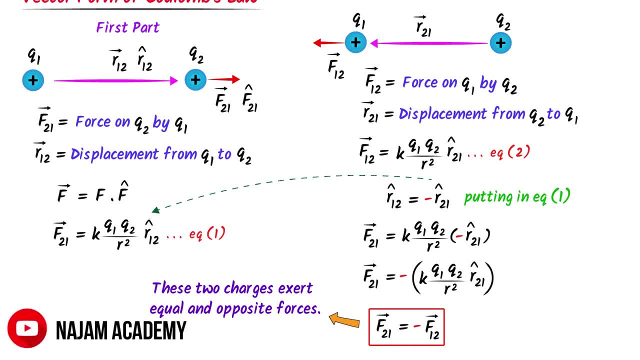 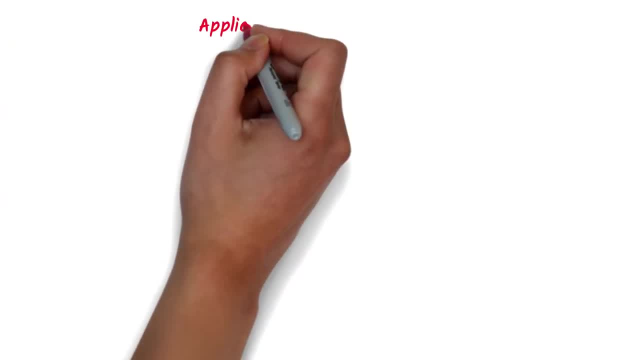 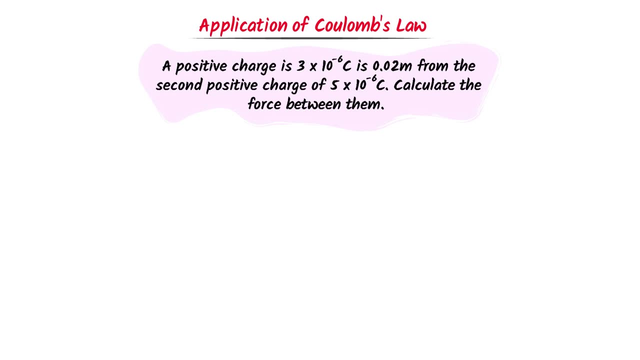 So this is the proof of writing Coulomb's law in vector form. So this is the proof of writing Coulomb's law in vector form. Finally, let me teach you the application, or numerical, of Coulomb's law. A positive charge of 3 into 10 to the power negative 6 Coulomb is 0.02 meter away from the second positive charge of 5 into 10 to the power minus 6 Coulomb. 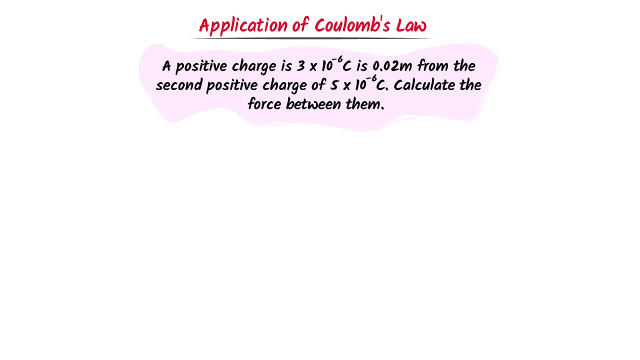 Calculate the force between them. Well, firstly I write the given data. Let: the Q1 charge is 3 into 10 to the power minus 6 Coulomb. The Q2 charge is 5 into 10 to the power minus 6 Coulomb. 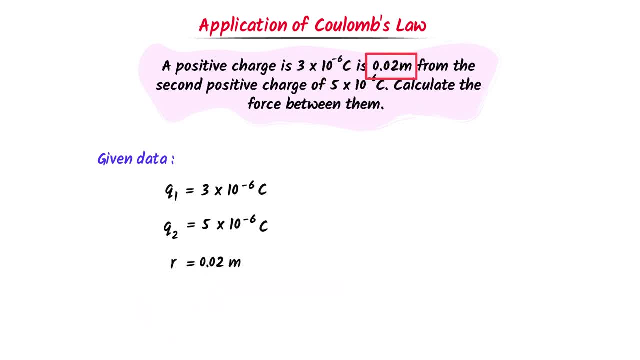 The distance between them is 0.02 meter and the force between them is required. We know that, using Coulomb's law, we can calculate the force between them. I write: F is equal to K into Q1. Q2 upon R squared into R21 hat. 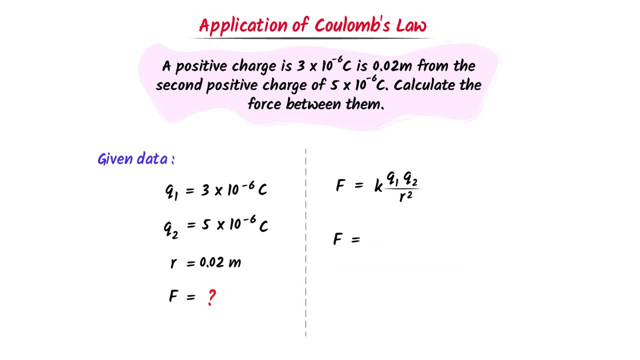 R, F is equal to the value of K, is 9 into 10, to the power 9, and I plug in all these values in this equation. After calculation I get: F is equal to 337.5 Newton, So the force between charges is 337.5 Newton. 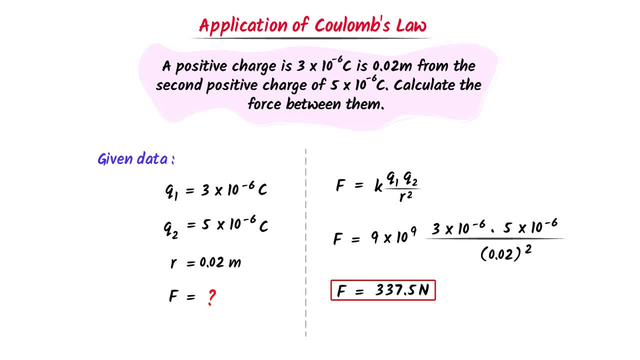 Therefore, using Coulomb's law, we can calculate Coulomb's force between charge. This was all about Coulomb's law.